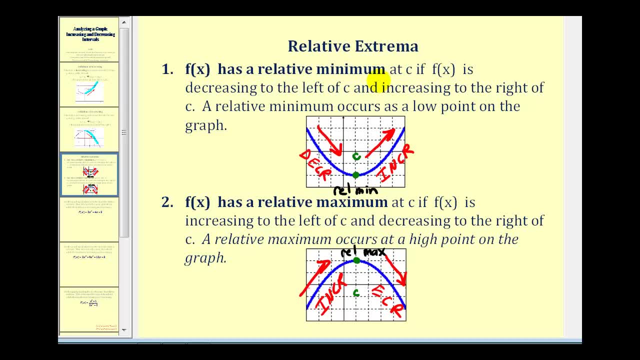 where a function changes from increasing to decreasing or from decreasing to increasing, So the function will have a relative minimum, pictured here at x equals c. if the function changes from decreasing to increasing, And the function will have a relative maximum, pictured here at x equals c. 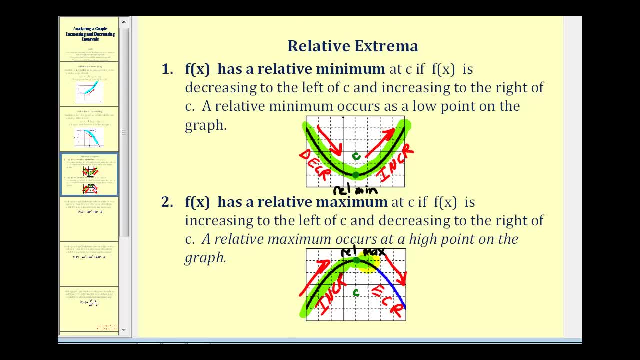 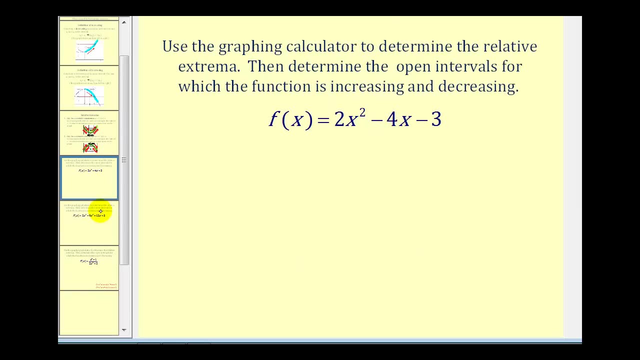 if the function changes from increasing to decreasing at x equals c. So we have a relative minimum at a low point on the graph and we have a relative maximum at a high point on the graph. So let's go ahead and take a look at an example. Here we want to use the graphing calculator to 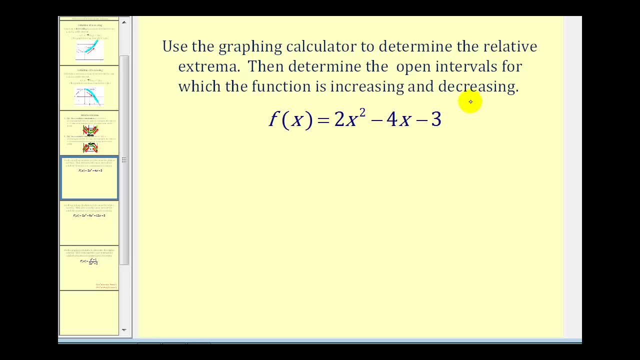 determine the relative extrema and then determine the open intervals for which the function is increasing and decreasing. The first thing we should recognize here is that we have a polynomial function or more specifically a quadratic function, And therefore the domain for this function would be all real numbers. 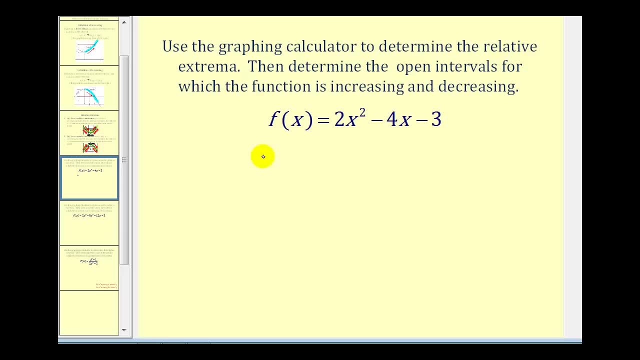 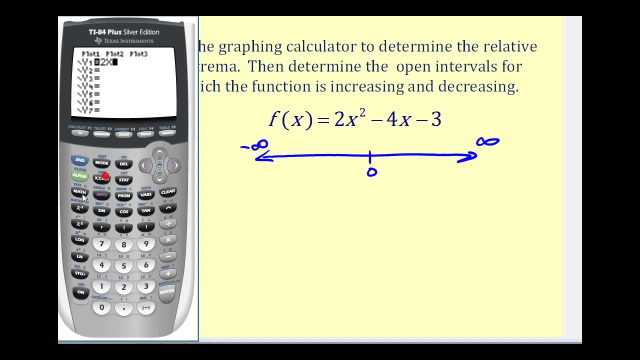 So let's go ahead and sketch a number line that would show the domain of this function. So we would have from negative infinity all the way to positive infinity. Now let's go ahead and graph this on our graphing calculator. So we're going to press y equals type in our function. 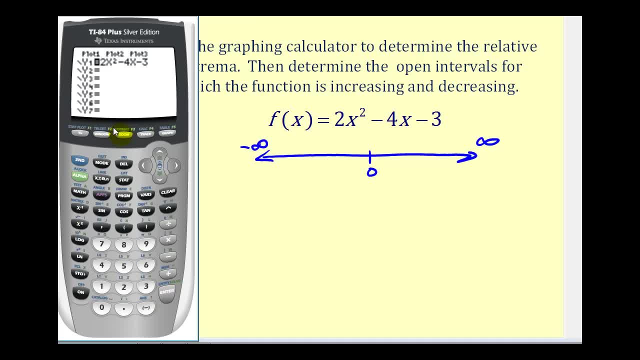 let's go ahead and press zoom six to make sure we have the standard window. By analyzing the graph, we can see that it decreases on this interval. then we have a low point and then the function starts to increase. So because we have a low point here, we have a relative minimum. 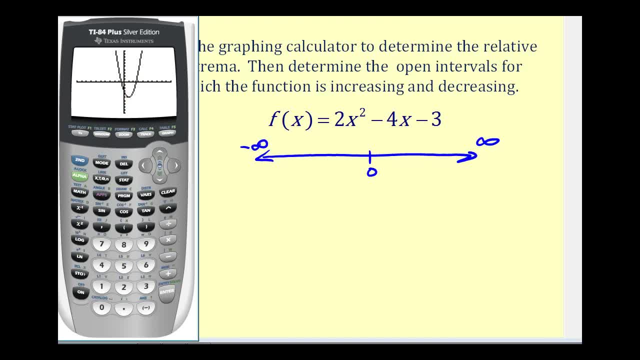 let's go ahead and find that first. So we're going to press second trace, select the minimum option. it's asking us to be to the left side of the relative minimum and we are, but let's go ahead and get a little bit closer. 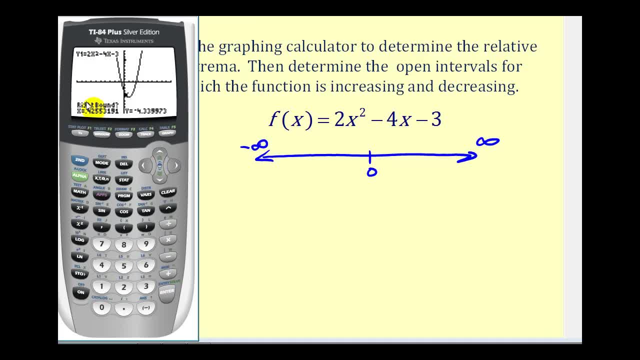 Let's press enter. it's going to ask for the right bound. we'll move to the right side of the minimum point, maybe somewhere in here. press enter. When it asks us to guess, let's go ahead and move the cursor closer to the actual minimum. 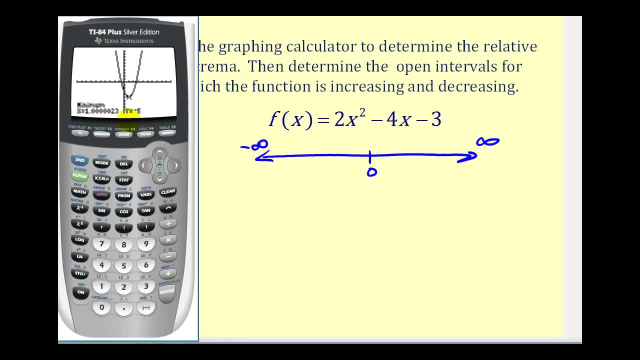 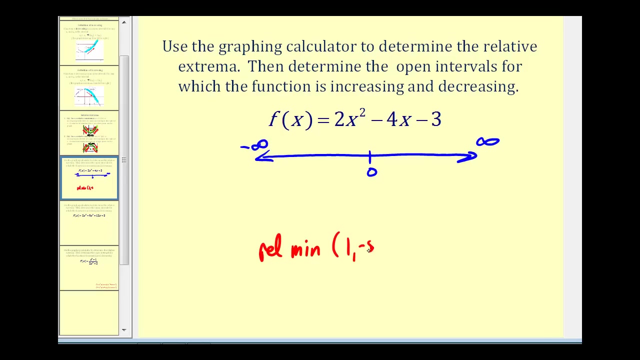 value which is here. So the point one negative five represents the relative minimum. And then notice: to the left of that point the function is decreasing and to the right it is increasing. Let's go ahead and write this information down. The relative minimum occurs at the point one negative five. 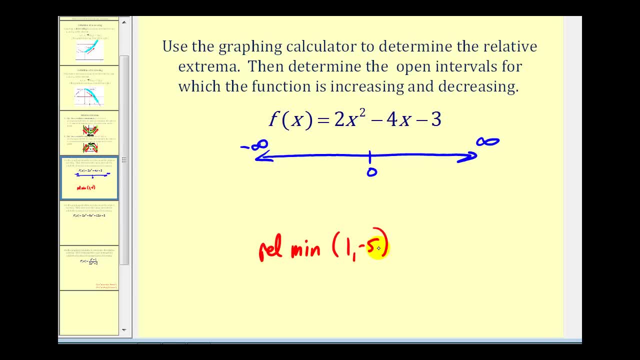 Some texts like to identify the relative minimum as an ordered pair, but remember that the x coordinate is the location and the y coordinate is actually the minimum value. So we could give the same information by saying that at x equals one, the relative minimum. 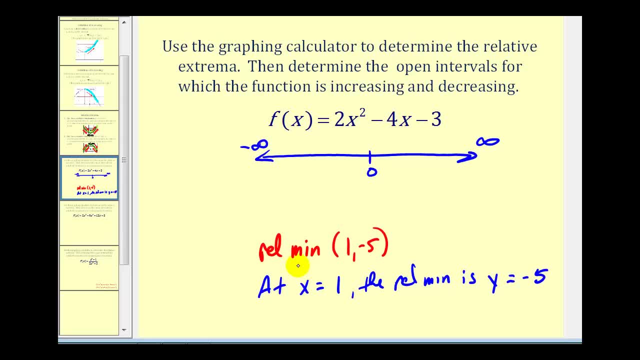 is y equals negative five. Now, since we know that the function changes from decreasing to increasing at x equals one, we're going to go ahead and use that point to help us determine the intervals for which the function is increasing or decreasing. So a positive one will make an open circle, because the question asked for the open intervals for 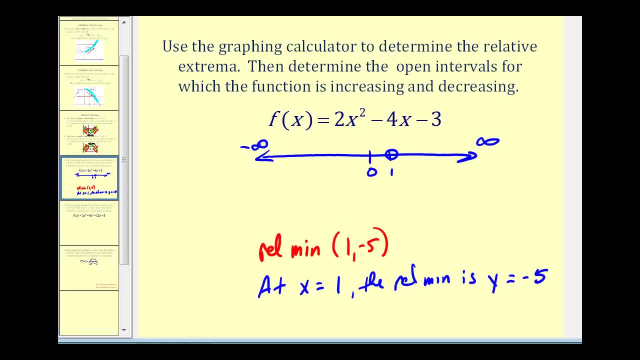 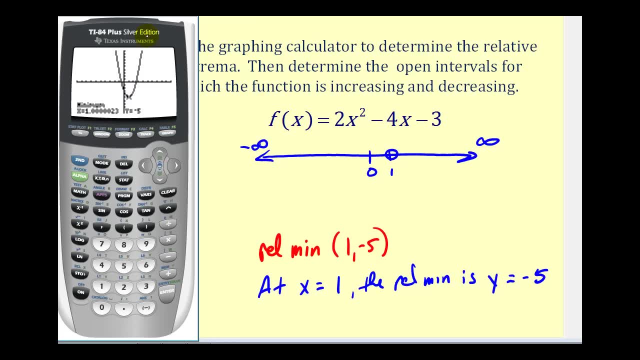 at which the function is increasing and decreasing. So let's go back and look at the graph again: To the left of one, the function is decreasing, and to the right of positive one, the function is increasing. So it's decreasing on this interval. 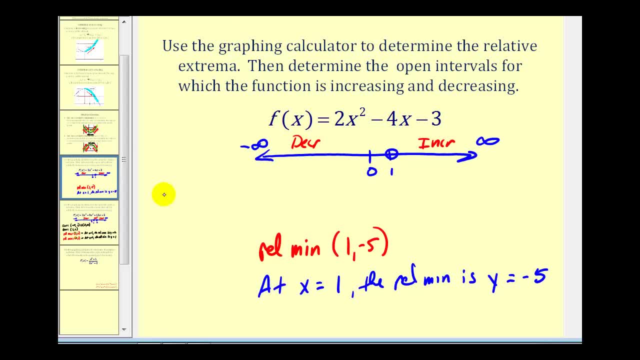 and increasing on this interval. Let's go ahead and write that out: It's decreasing on the interval from negative infinity to positive one and it's increasing on the interval from one to positive infinity. So if we graph the domain of the function, 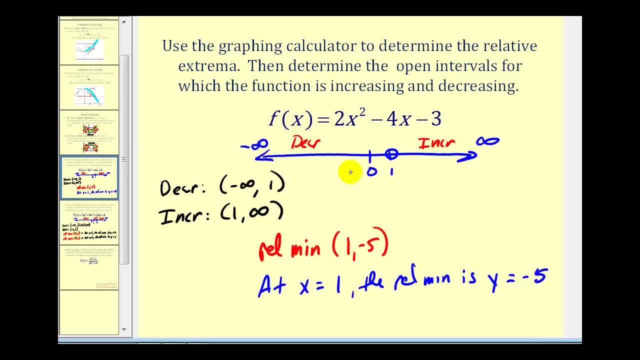 then plot the locations of any relative extrema on the graph of the domain. it'll help us determine the intervals for which the function is increasing and decreasing. Let's go and take a look at our second example. It's the same question. We want to determine the relative extrema. 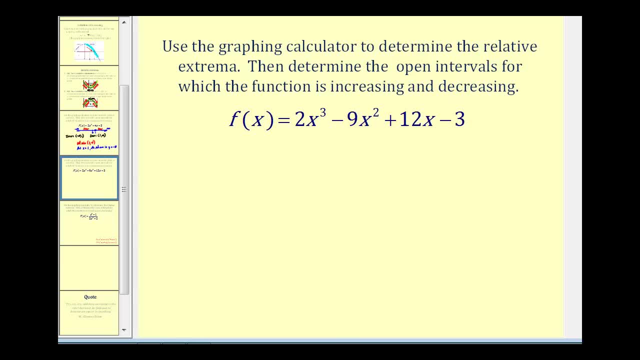 and then the intervals for which the function is increasing and decreasing. So we should recognize this as a polynomial function or more specifically a cubic function, and the domain would be all real numbers. So we have to consider the numbers from negative infinity to positive infinity. 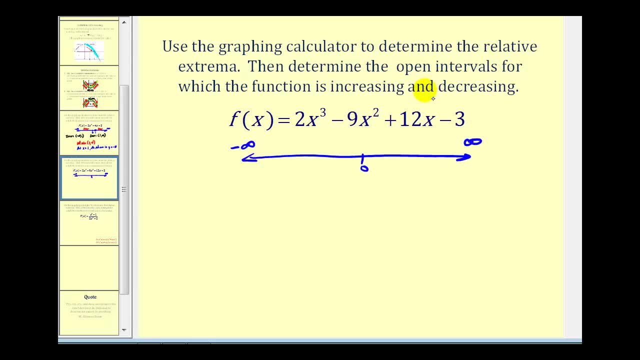 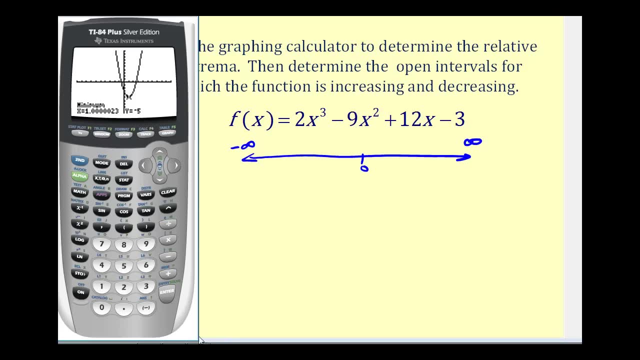 when determining the intervals for which the function is increasing and decreasing. Let's go ahead and graph the function and identify the relative extrema Press y equals. clear this function out and enter the new function: Press graph. Press graph: We can see it's increasing, decreasing and then increasing. 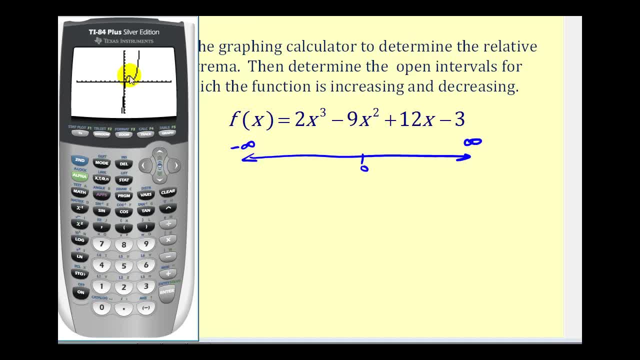 and it changes at this high point tier and this low point tier. This high point tier represents a relative maximum And this point here represents a relative minimum. Let's go ahead and zoom into this area to get a closer look at the function in this region here. 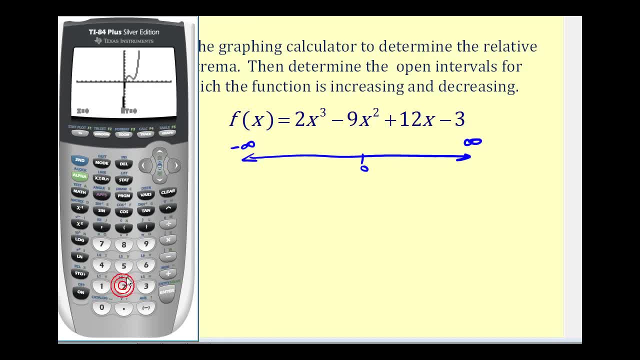 So we'll press zoom option two: We're going to move this blinking pixel closer to the area that we want to zoom into. So I'm going to go to the right and then move up a little bit. Then, from here, I'll press enter. 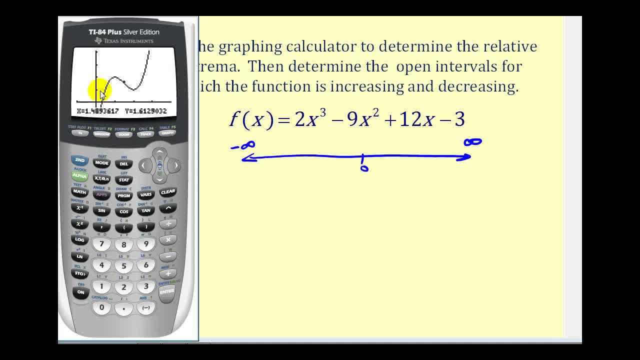 And now we have a much better view of the graph, where it changes from increasing to decreasing and then back to increasing. Let's go ahead and find this point here. that represents the relative maximum. So we'll press second trace for the calculation menu and then press option four for maximum. 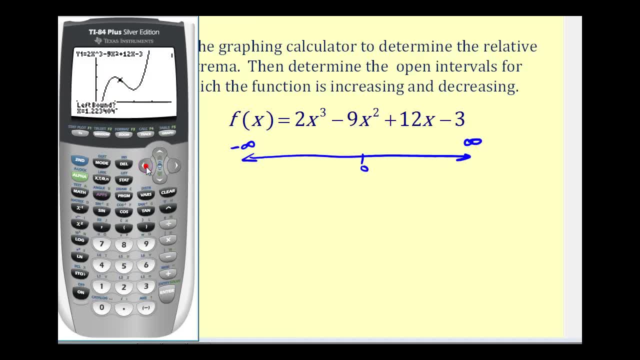 We need to be to the left side of this high point. so we'll press the left arrow until we're to the left side of the hill Press: enter. Move to the right side of the high point of the hill Press. enter When it says guess, we're going to move the cursor. 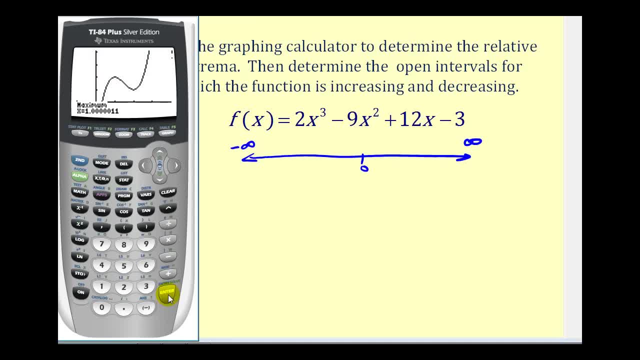 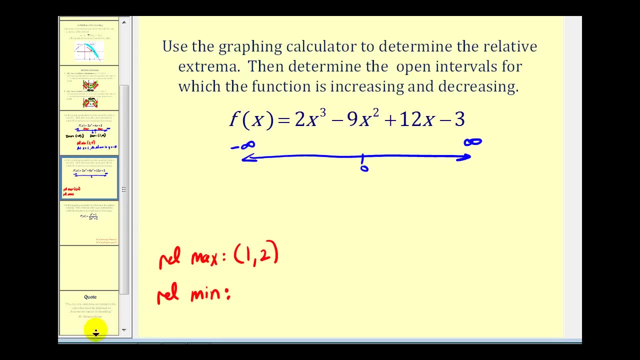 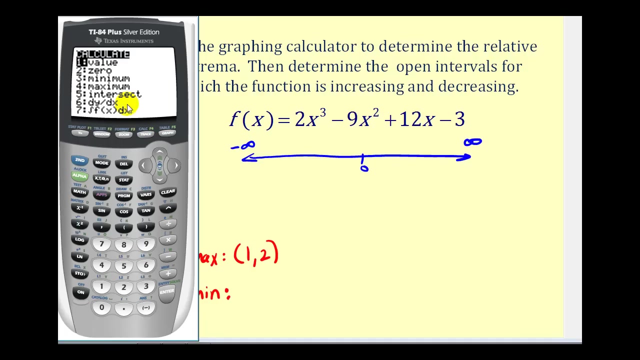 closer to the actual maximum. Press enter: And this relative maximum is the point one. two: Let's go ahead and write that down. Now let's find the relative minimum. We're going to press second trace again. Option three for minimum. 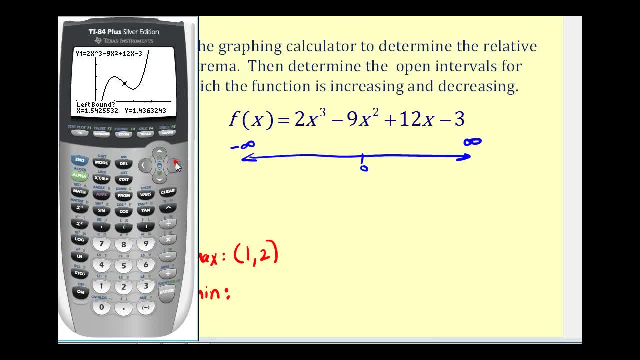 Let's move closer to the low point, but remain on the left side Somewhere in here, Press enter. Move to the right side of the minimum, Press enter, Move a little bit closer and then press enter again And the relative minimum would be the point two one.